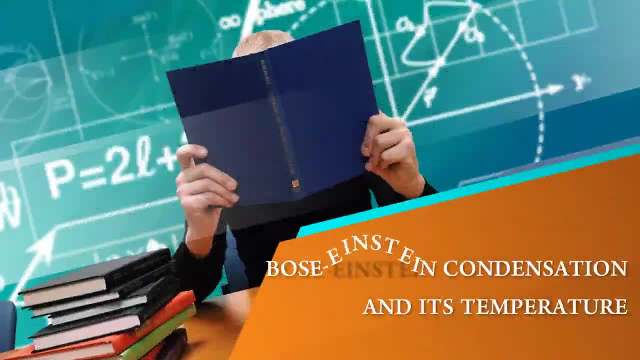 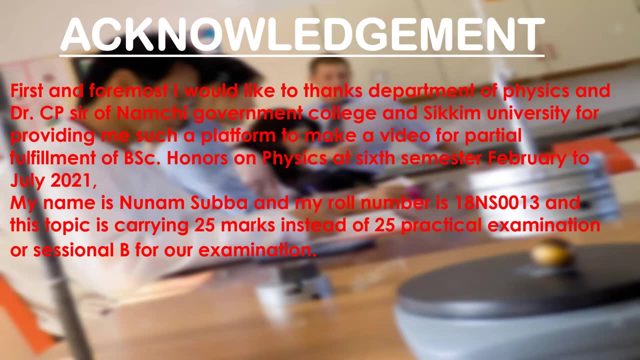 Acknowledgement. First and foremost, I would like to thank Department of Physics and Dr Sipi Sir of Namjee, Gowmin College and Sikkim University for providing me such a platform to make a video for partial fulfillment of PSE honors on physics at 6th semester, February. 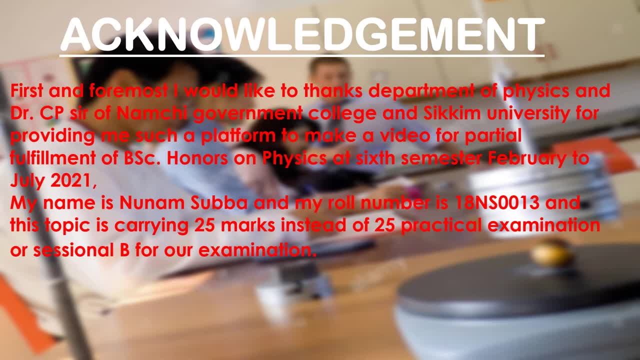 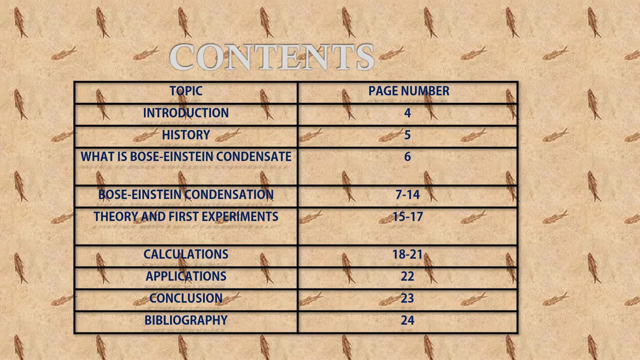 to July 2021.. My name is Nunam Subba and my roll number is 18NS0013, and this topic is carrying 25 marks instead of 25: practical examination or sessional B for our examination. Contents, Topic and page number: Introduction: 4. History. 5. What is Bose-Einstein condensate? 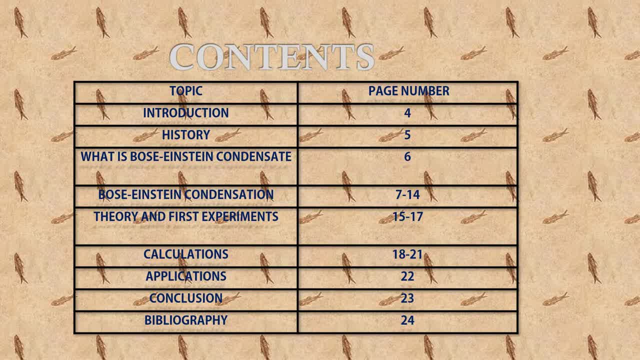 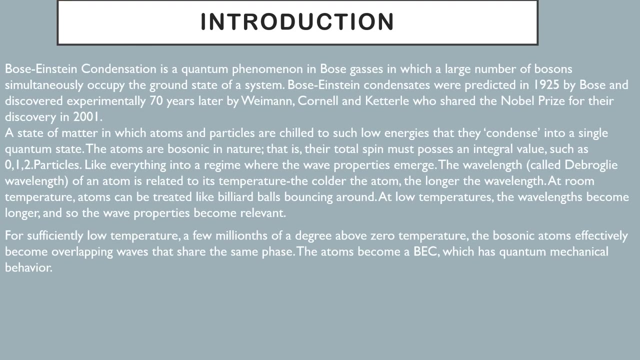 6. Bose-Einstein condensation: 7 to 14. Theory and first experiments: 15 to 17. Calculation: 18 to 21. Application: 22. Conclusion, 23. Bibliography Point 4. Introduction: Bose-Einstein condensation is a quantum phenomenon in Bose gases in which 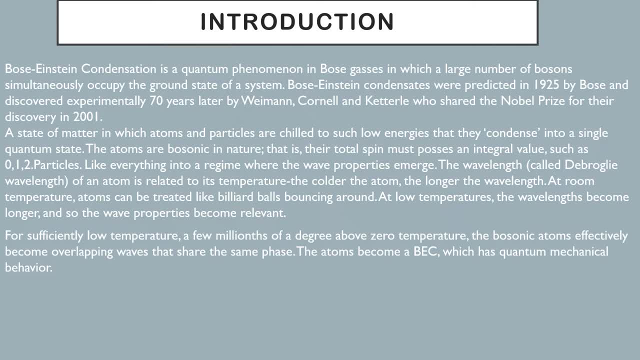 a large number of bosons simultaneously occupy the ground. state of a system. Bose-Einstein condensate was predicted in 1925 by Bose and discovered experimentally 70 years later by Wyman, Cornell and Catley, who share the Nobel Prize for the discovery in 2001.. A state 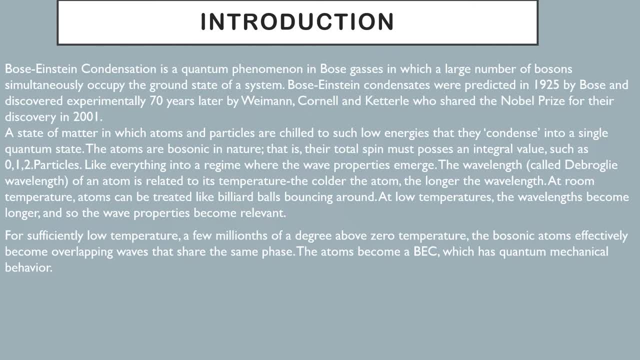 of matter in which atoms and particles are chilled to such low energies that they condensate into a single quantum state. The atoms are bosonic in nature, that is, their total spin must possess an integral value, such as 0,, 1, 2.. Particles, like everything else, are: 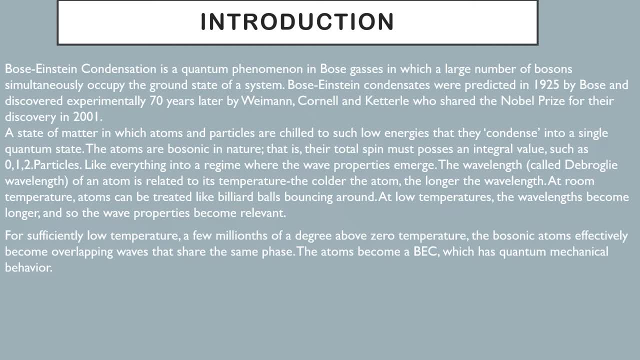 all in a rhythm where the wave properties emerge. The wavelength, called the three-Brooklyn wavelength, of an atom is related to its temperature. The colder the atom, the longer the wavelength. At room temperature atoms can be treated like billiard balls bouncing around At low. 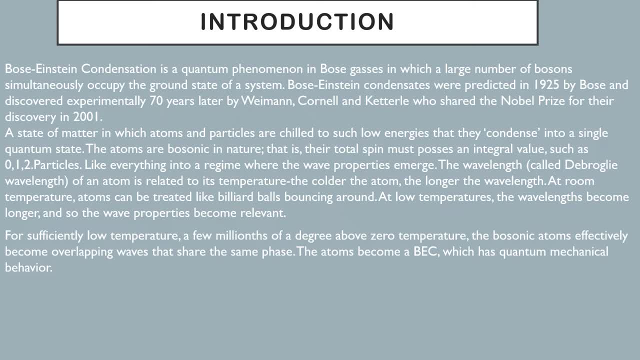 temperatures. the wavelengths become longer, and so the wave properties become relevant For sufficiently low temperature of few millions of a degree above zero temperature. the bosonic atoms effectively become overlapping waves that share the same phase. The atoms become a BSE, which has quantum mechanical behavior. 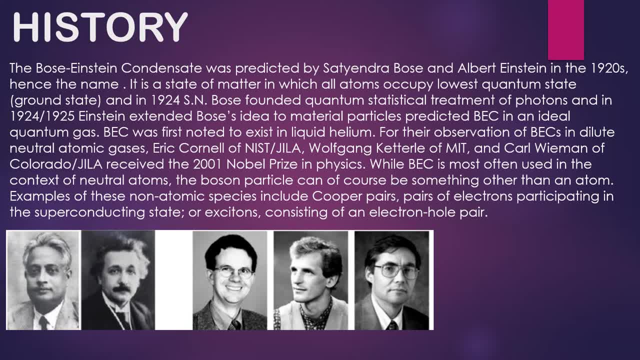 History. The Bose-Einstein condensate was predicted by Satyendra Bose and Albert Einstein in the 1920s, Hence the name. it is a state of matter in which all atoms occupy lowest quantum ground state, And in 1924, Assange-Bose founded quantum statistical treatment of photons and in 1924-1925, Einstein. 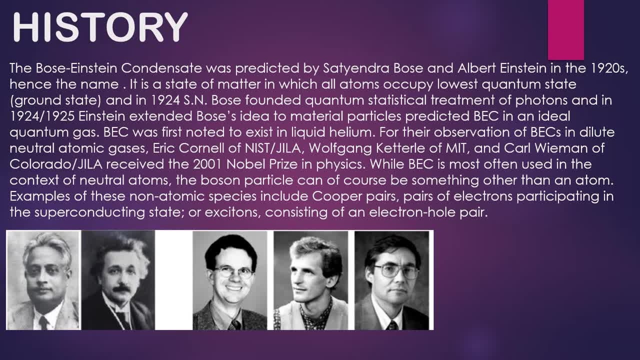 extended Bose's idea to Newton. He came up with the idea of quantum processing and the theory about quantum processing and the theory of quantum processing, in which we tend to refer to the synthesis of the quantum state. as quantum physics, BSE and ILS started in 1923.. 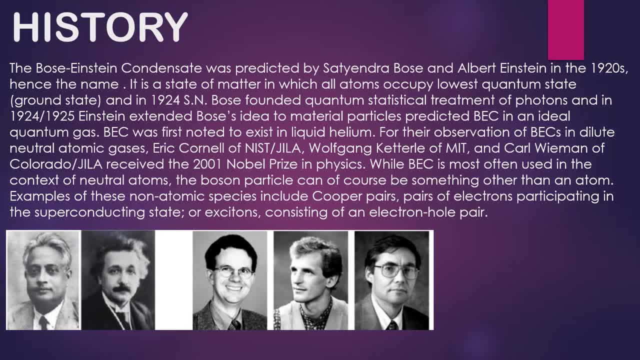 BSE is a quantum building and it was the first low-power quantum building. We saw that there is much more understanding of quantum physics than there is in quantum physics. BSE is a quantum building and it has a very large capacity to cultivate and convert quantum. 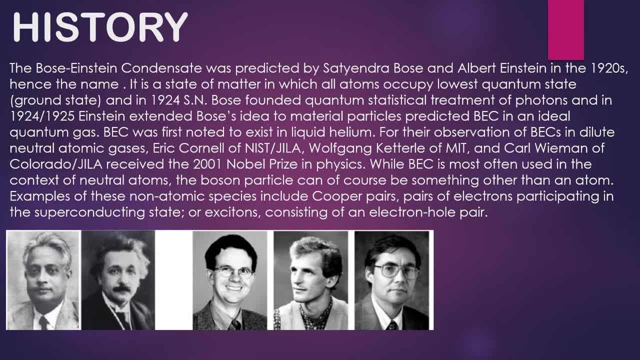 particles in very small amounts, We saw that there is very much more understanding of quantum physics. The Jazz pushing the power of quantum physics is not a matter of a particle, but of a matter of energy. But it is a matter of money. It is a matter of money. 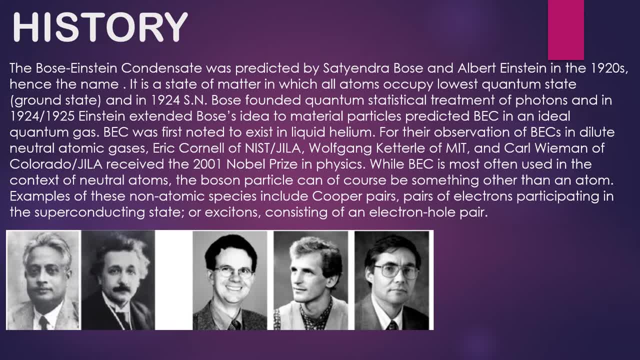 And it can be used for any use of energy, of technology. It changes its shape and calls for the change of energy. Wolfgang Catterley of MIT and Carr Women of Colorado received the 2001 Nobel Prize in Physics. While BEC is most often used in the content of neutral atoms, the boson particles can 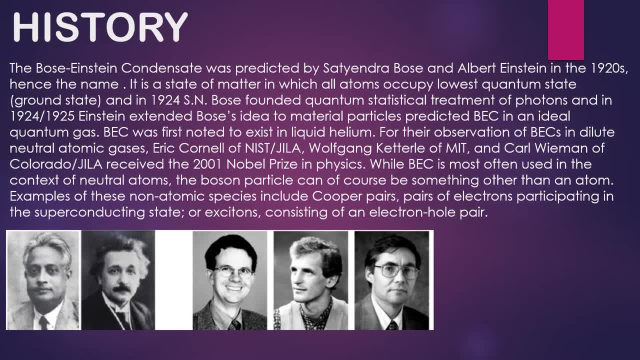 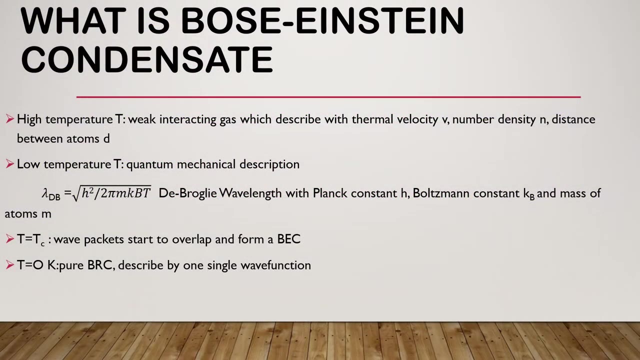 of course, be something other than an atom. Examples of these non-atomic species include copper pairs, pairs of electrons participating in the superconducting state, or excitons consisting of an electron-hole pair. What is Bose-Einstein condensate? High-temperature, weak interaction gas which is described with thermal. 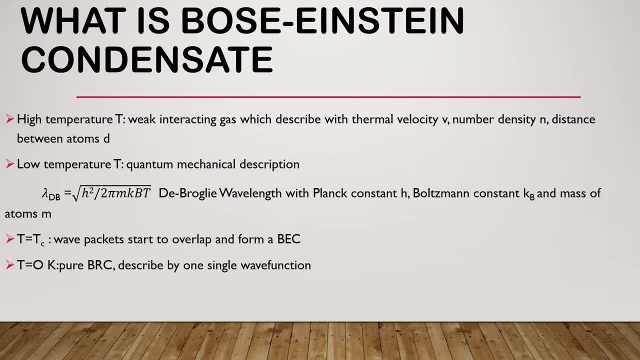 velocity, Velocity v, number, density n, distance between atoms d, Low-temperature t. quantum mechanical description: Lambda db equals to: under root h, square slash 2, pi, mk, Bt, d, Broccoli wavelength with Planck constant h, Boltzmann constant kb and mass of the. 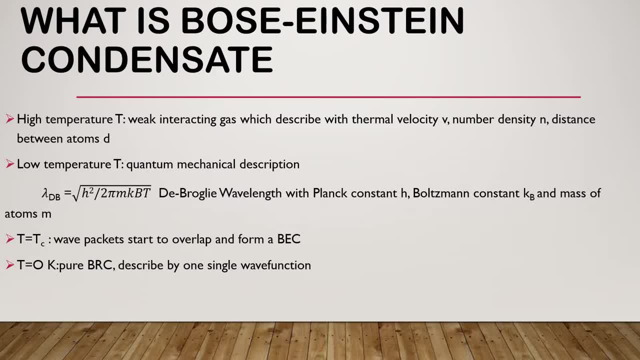 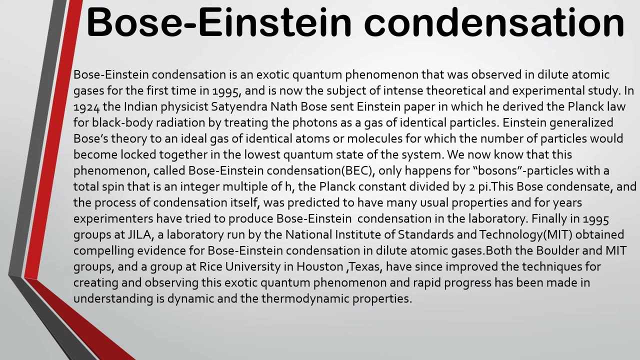 atoms m. T equals to Tc. wave packets start to overlap and form a BEC. t equals to 0 k pure Brc described by one single wave function: Bose-Einstein condensation. Bose-Einstein condensation is an exotic quantum phenomenon that was observed in the early 20th century. 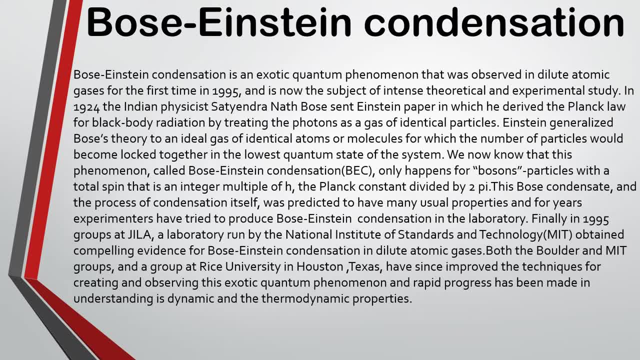 It was observed in dilute atomic gases for the first time in 1995 and is now the subject of intense theoretical and experimental study. In 1924, the Indian physicist Satyendra Nadebo sent Einstein a paper in which he derived the Planck constant for blackbody radiation by treating the photons as a gas of identical. 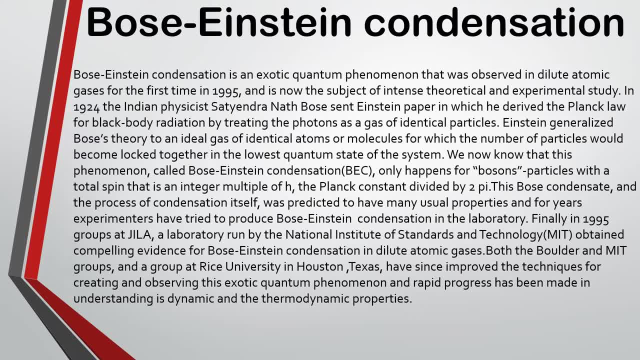 particles. Einstein generalized Bose theory to an ideal gas of identical atoms or molecules, for which the number of particles would become locked together in the lowest quantum state of the system. We know that this phenomenon, called Bose-Einstein condensation, BEC, only happens for a boson particle with a total spin that is an integral multiple of h. 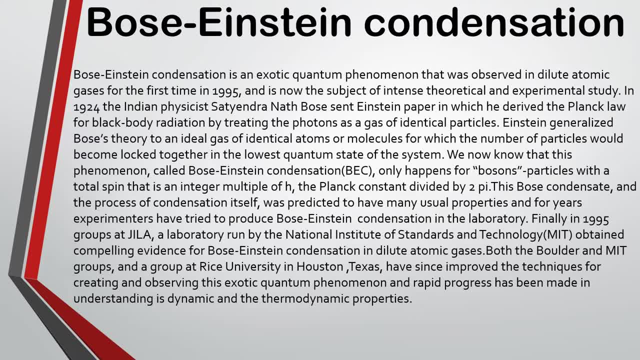 The Planck constant divided by 2 pi. this Bose condensate and the process of condensation itself was predicted to many users. For years, experimenters have tried to produce Bose-Einstein condensation in the laboratory. Finally, in 1995, groups at JILA, a laboratory run by the National Institute of Standards and Technology, obtained compiling evidence for Bose-Einstein condensation in dilute atomic gases. 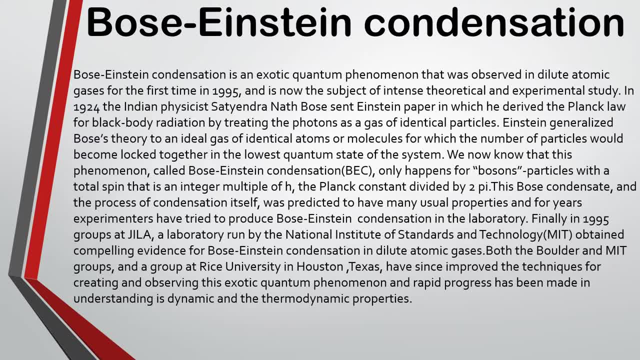 Both the Boulder and MIT labs conducted experiments. Both the Boulder and MIT labs conducted experiments. Both the Boulder and MIT labs conducted experiments. The goal is to repeat this method pressed into our mass today. The goal is also to convert it into long key cosmological data in the future to 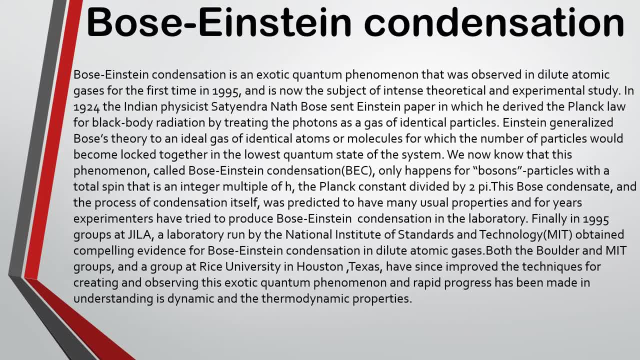 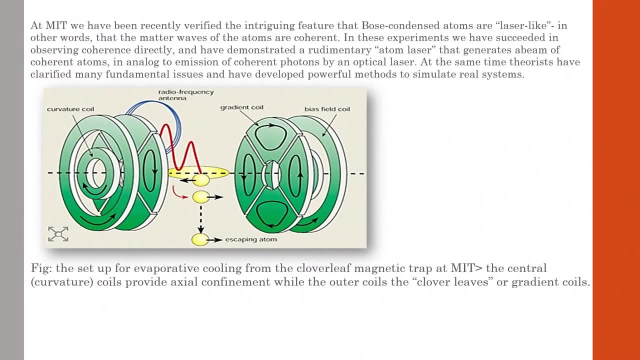 Institutions also expect to implement this method. We are excited to see what our future projects will look like And we are excited to see what other research projects we are approaching in the future. Thank you for watching this video. Goodbye everyone. the features that both condensed atoms are laser-like, in other words, that the matter. 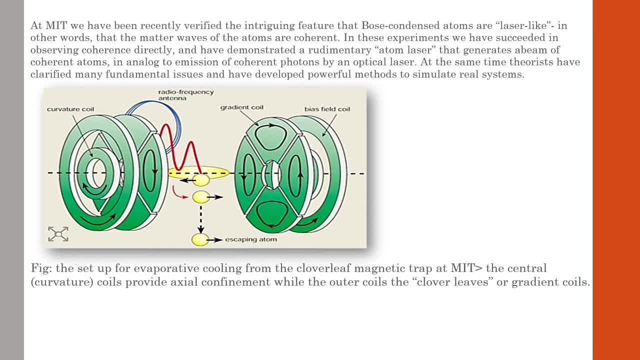 waves of the atoms are coherent. In this experiment, we have succeeded in observing coherence directly and have demonstrated a rudimentary atom laser that generates a beam of coherent atoms in analog to emission of coherent photons by an optical laser. At the same time, theorists have clarified many fundamental issues and have developed 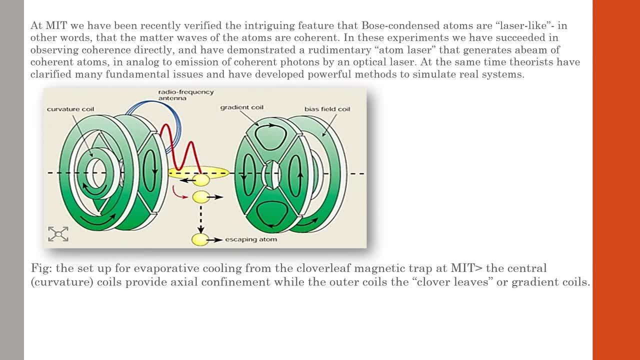 powerful methods to stimulate real systems. We can see the figure: The set-off for evaporative cooling from the Cloverleaf magnetic trap at MIT. the center curvature coils provide action, The radial confinement, while the other coil, the Cloverleafs, are gradient coil. 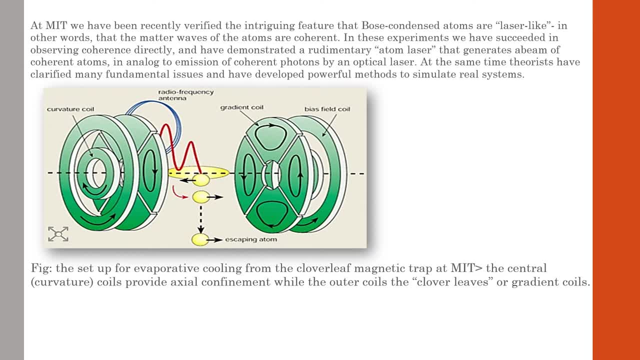 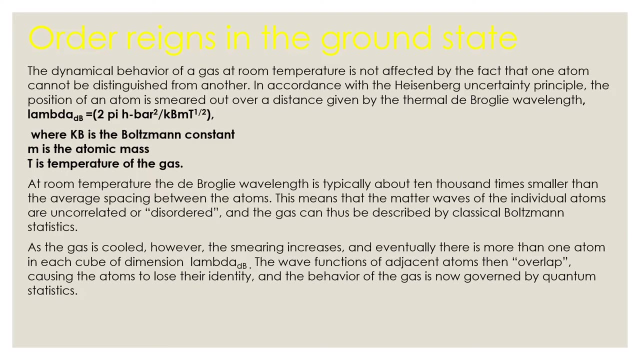 And there we can see bias-filled coil radio-frequency antenna escaping atoms Other range in the ground state. The dynamical behavior of a gas at room temperature. At room temperature is not affected by the fact that one atom cannot be distinguished from another. In accordance with the Heisenberg uncertainty principle, the position of an atom is smudged. 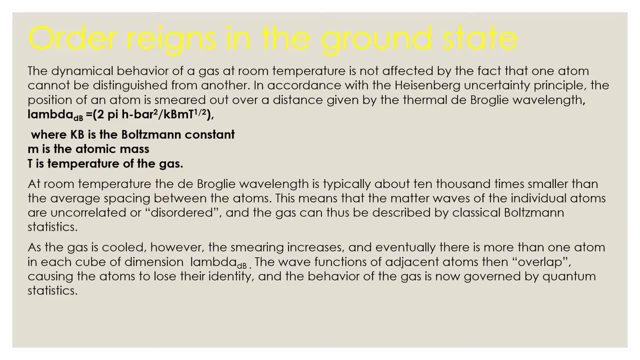 out over a distance by the given thermal de Broglie wavelength Lambda. db equals to 2 pi h bar square by kb mt to the power half, Where kb is the bulk. So kb is the mass. The mass is the Bozeman constant. 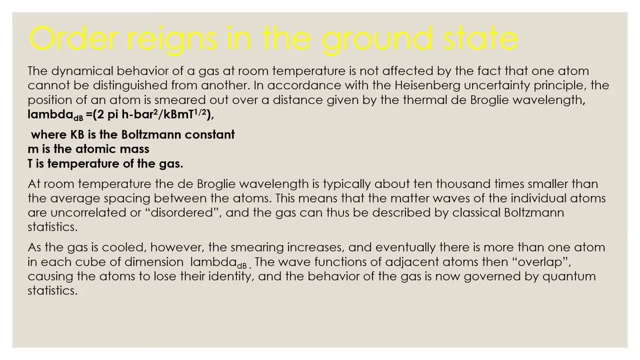 M is the atomic mass. T is the temperature of the gas. At room temperature, the de Broglie wavelength is typically about 10,000 times smaller than the average spacing between the atoms. This means that the matter waves of the individual atoms are uncorrelated or disordered. 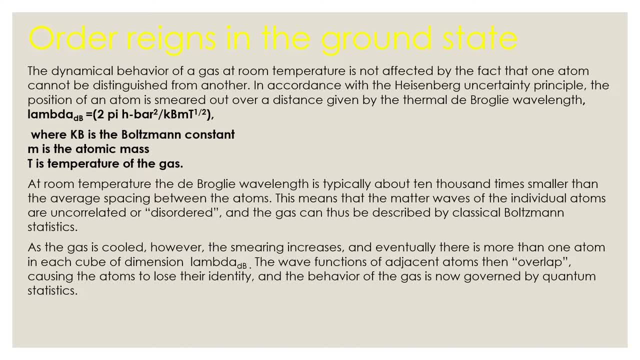 And the gas can thus be described by classical Bozeman statistics, As the gas is the mass of the atom. The mass of the atom is the mass of the atom. The mass is the temperature of the atom. The mass of the atom is supposed to be respect. The mass of the 말씀드� substance of the cosmos on the planet cannot be the same as the mass of fill, but the mass of the atom has to be equal to the mass of the atom. We can use Bayh-Hull's dimensioning. 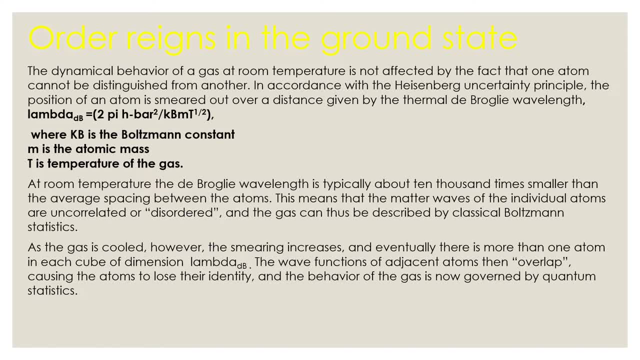 The mass of the atom is small, but frinea- The mass of a gas, is cold. However, the smoothing increases and eventually there is more than one atom in each cube of dimension. lambda db. The wave function of adjacent atoms then overlap, causing the atoms to lose their identity and 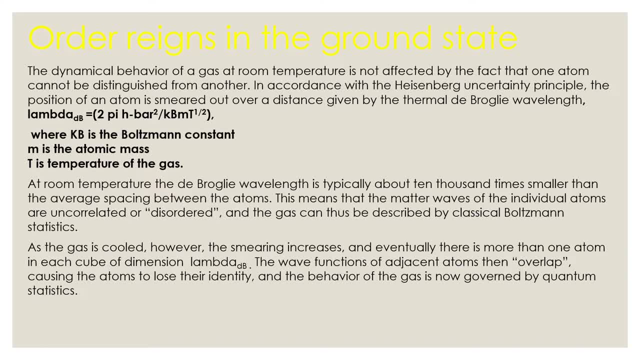 the behavior of the gas is now governed by quantum statistics. Now for the curved supper: K2, nu, k2, Mcineta, mgj. m. isno응e形 a ピmikal ðHm1巴1ω Π⋕t. 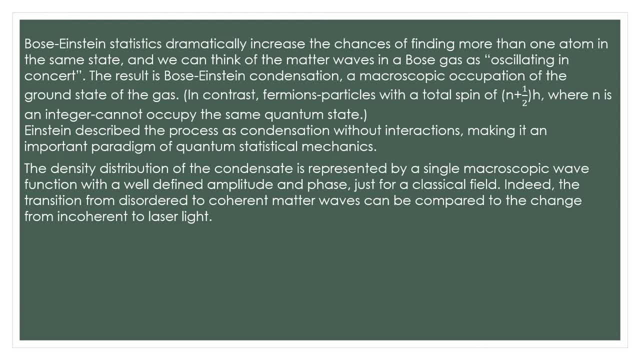 Bose-Einstein statistic dramatically increases the chances of finding more than one atom in the same state, and we can think of the matter waves in a Bose gas as oscillating in concert. The result is Bose-Einstein condensation, or microscopic occupation of the ground state. 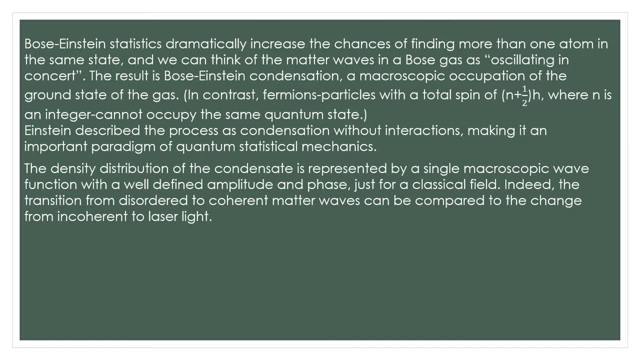 of the gas in contracts for muons, particles with a total spin of n plus 1 by 2 h, where n is an integer, cannot occupy the same quantum state. Einstein described the process as condensation without interaction, making it an important paradigm of quantum statistical mechanics. 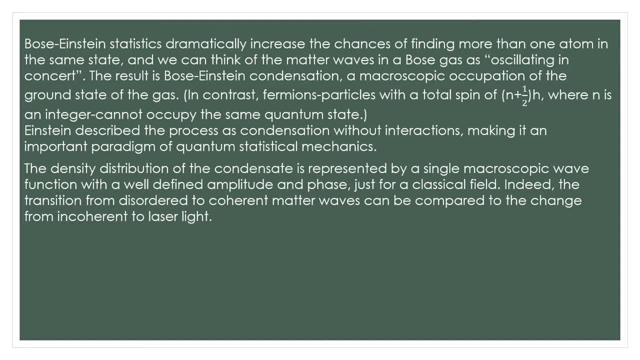 The density distribution of the condensate is represented by the density distribution of a single macroscopic wave functioned with a well-defined amplitude and phase, Just for a classical field. indeed, the transition from this order to coherent matter waves can be compared to the change from incoherent to laser light. 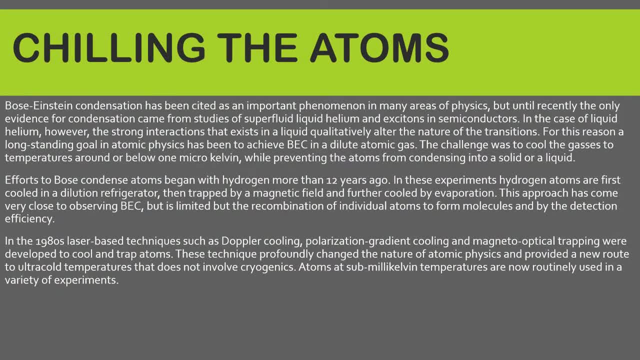 Chilling the Atoms. Bose-Einstein condensation has been cited as an important phenomenon in many areas of physics, but until recently, the only evidence for condensation came from studies of superfluid liquid helium and excitons in semiconductors. In the case of liquid helium, however, the strong interaction that exists in a liquid 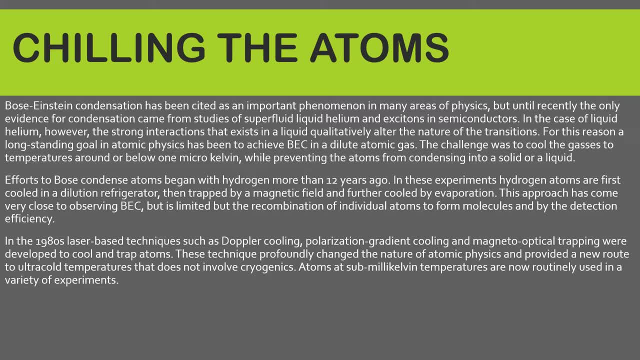 qualitatively alter the nature of the transition. The result: os these reasons, a longstanding goal in atomic physics have been to achieve base C in a dilute atomic gas. The challenge was to cool the gases to temperatures below one micro Lewis nationalism. 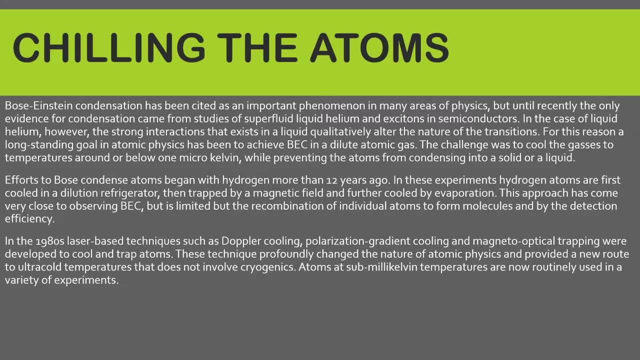 & around or below 1 micro Kelvin, while preventing the atoms from condensing into a liquid or a solid. 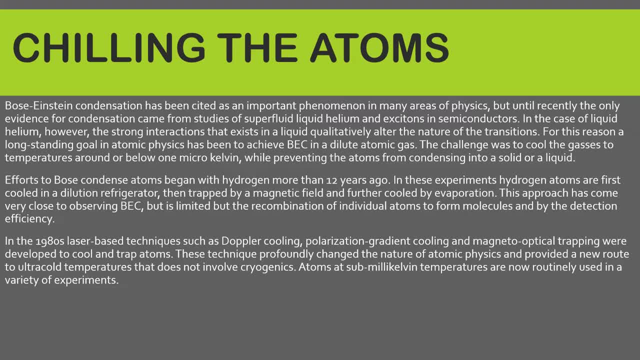 Efforts to Bose condensate atoms began with hacec hydrogen more than 12 years ago. In this experiment, hydrogen atoms are first cooled in a dilution refrigerator, then trapped by a magnetic field and further cooled by evaporation. This approach has been very close to observing BEC, but is limited by the recombination of. 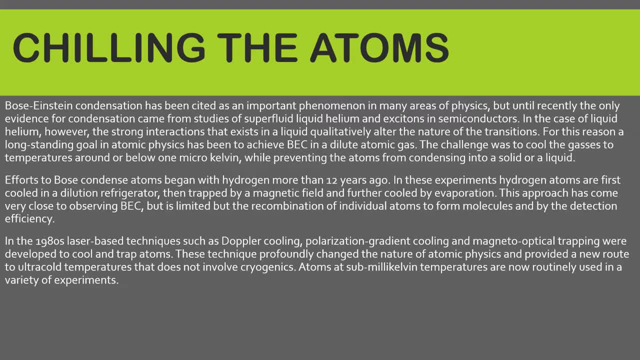 individual atoms to form molecules and by the detection efficiency. In the 1980s, laser-based techniques such as Doppler cooling, polarization gradient cooling and magneto-optical trapping were developed to cool and trap atoms. This technique profoundly changed the nature of 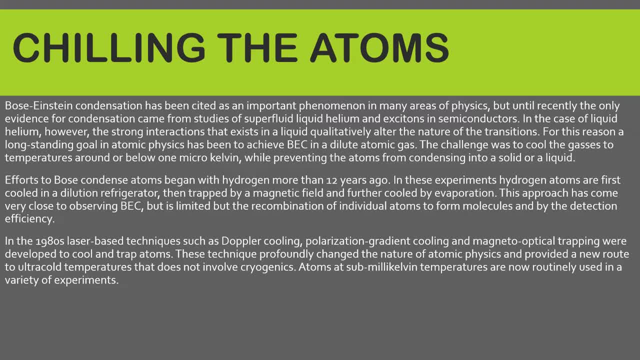 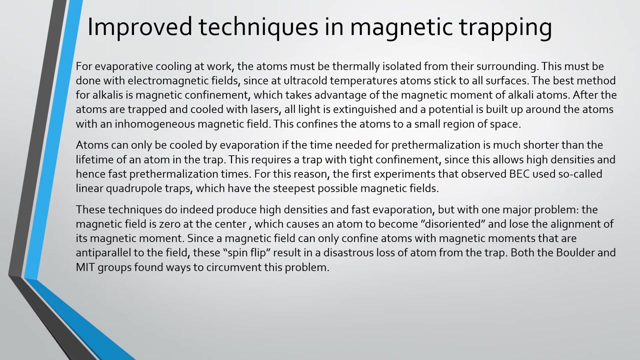 atom physics and provided a new route to ultra-cold temperature that does not involve cyclogene. Atoms at sub-milli-Kalvin temperatures are now routinely used in a variety of experiments. Improved Techniques in Magnetic Trapping For evaporative cooling. at work the atoms must be thermally isolated from the surroundings. 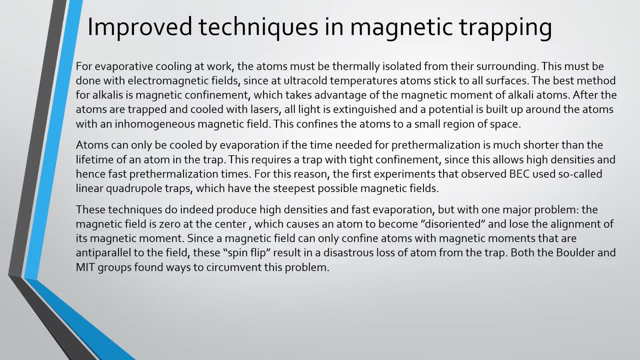 This must be done with electromagnetic fields, since at ultra-cold temperatures atoms stick to all surfaces. The best method for alkyl is magnetic confinement, which takes advantage of the magnetic movement of alkyl atoms. After the atoms are trapped and cooled with lasers, all light is extinguished and a potential is built up around the atoms with an inhomogeneous 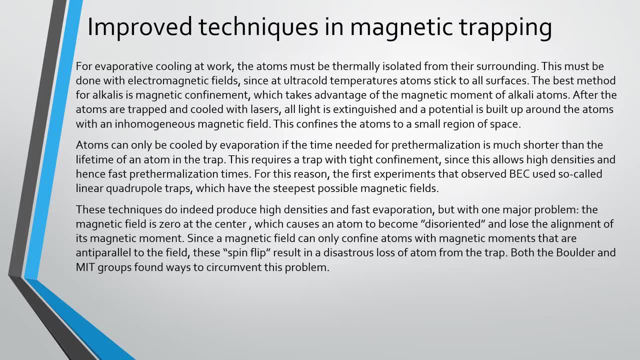 magnetic field. This confines the atom to small region of space. Atoms can only be cooled by evaporation if the time needed for pre-thermalization is much shorter than the lifetime of an atom in the trap. This requires a trap with tight confinement, since these allow high densities. 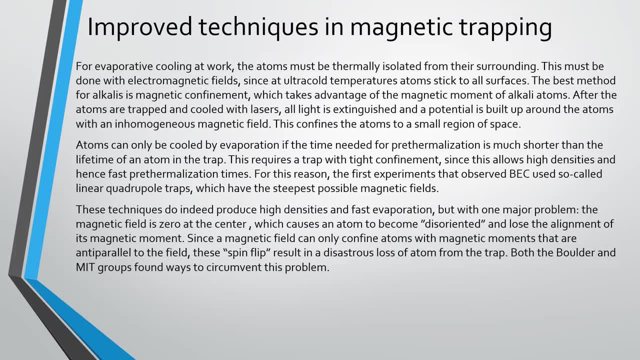 and hence fast pre-thermalization times. For this reason, the first experiment that observed BC used so-called linear quadrupole traps, which have the steepest possible magnetic fields. This technique do indeed produce high density and fast evaporation, but with one major problem. 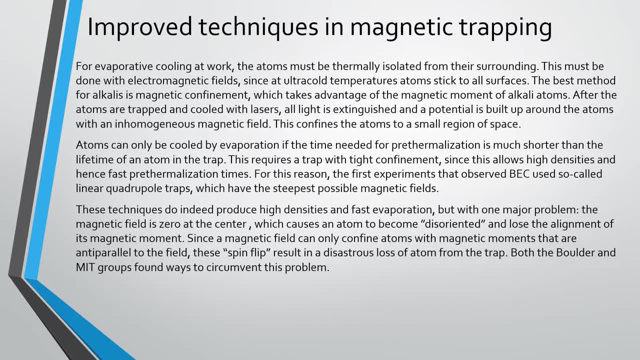 the magnetic field is zero at the center, which cause an atom to become disoriented and lose the alignment of its magnetic moment. Since a magnetic field can only confine atoms with magnetic moments that are anti-parallel to the field, this spin flip result in a distortious loss of atoms from. 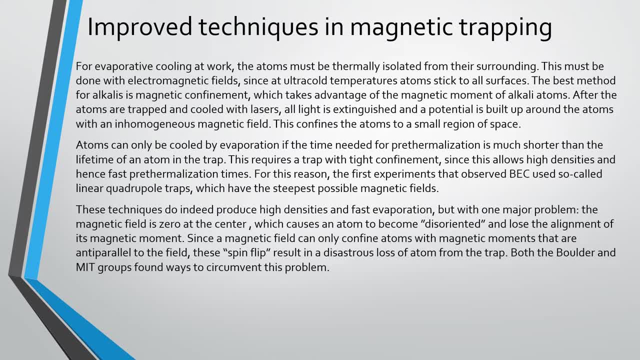 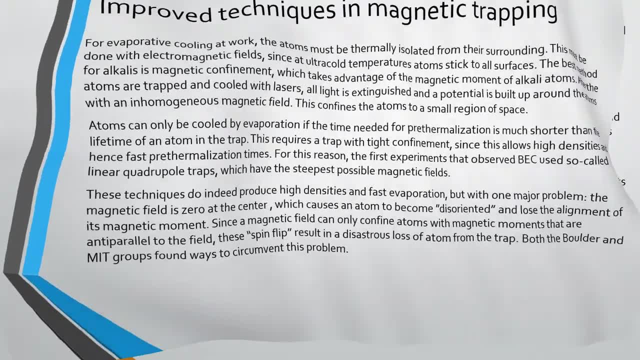 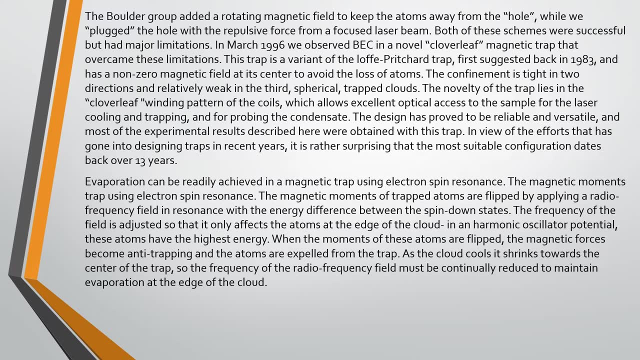 the trap. Both the border and MIT groups found ways to circumvent this problem. Since the whole of Earth was rock-solid, it was difficult to configure the rotation of the atom in traversing the magnetic field. The border group added a rotating magnetic field to keep the atoms. 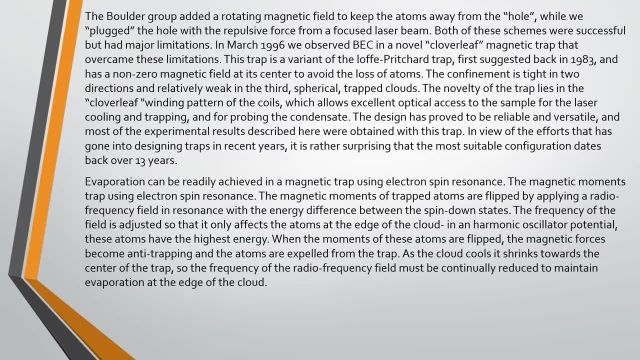 away from the whole, While we plugged the hole with a repulsive force from a focused laser beam. both of the schemes were successful but had major limitations. In March 1996, we observed BC in a novel cloverleaf magnetic field trap that overcame this limitation. This trap is a variant of the Lofi pre-chart trap. first, 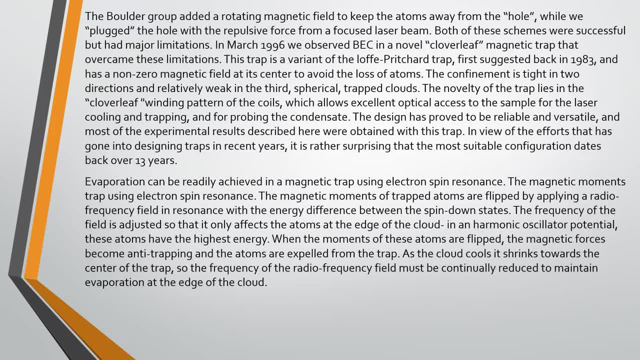 suggested back in 1983, and has a non-zero magnetic field at its center to avoid the loss of atoms. The confinement is tight in two directions and relatively weak in the third Spherical trap clouds. The novelty of the trap lies in the global deep winding. 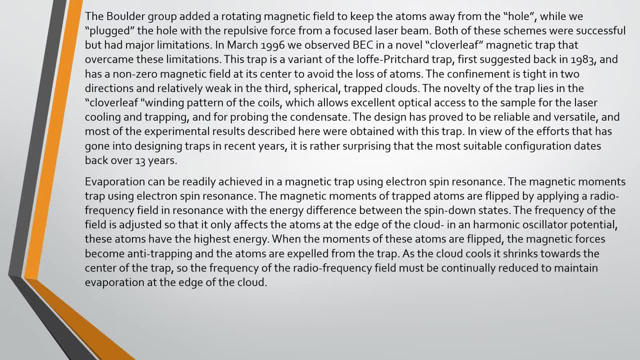 patterns of the coil, which allows excellent optical access to the symbol for laser cooling and trapping and for proving the condensate. The design has proved to be reliable and versatile, and most of the experimental results described here were obtained with this trap in view. 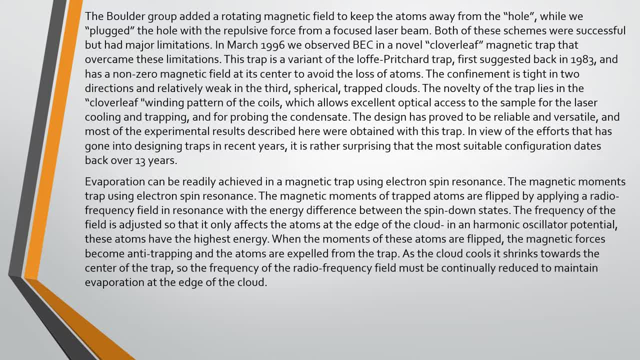 of the efforts that has gone into designing traps in recent years, it is rather surprising that the most suitable configuration dates back over 13 years. Evaporation can be readily achieved in magnetic trap using electron spin resonance: the magnetic moment trap. using electron spin resonance: The magnetic moment of trap. atoms are flipped by applying a radio. 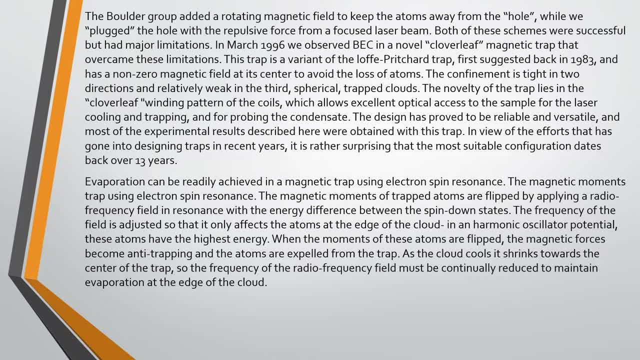 frequency field. in resonance, The magnetic moment of trap, atoms have the highest energy. when the moment of this atom are flipped, the magnetic force becomes anti-trapping and the atoms are expelled from the trap. As the cloud cools, it stings. When the magnetic force becomes anti-trapping, it just takes. 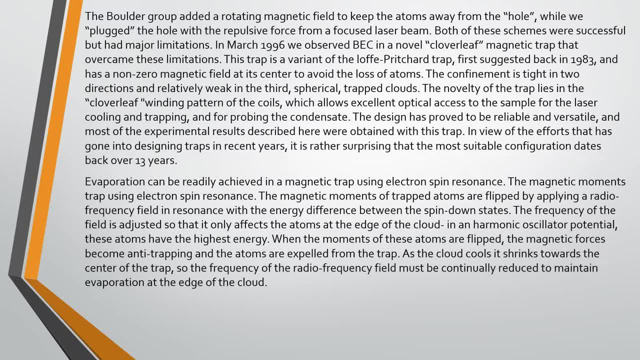 an extra strength to trap the atom into a Nathan Hemp 2 type atom. The magnetic force only affects the atom at the edge of the cloud in a harmonic oscillator potential, The magnetic towards the center of the trap. so the frequency of the radio frequency field must be continually. 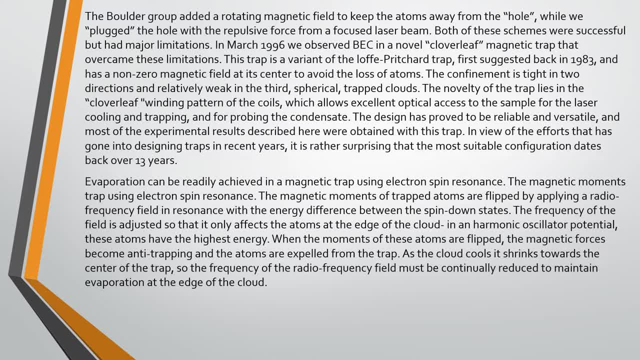 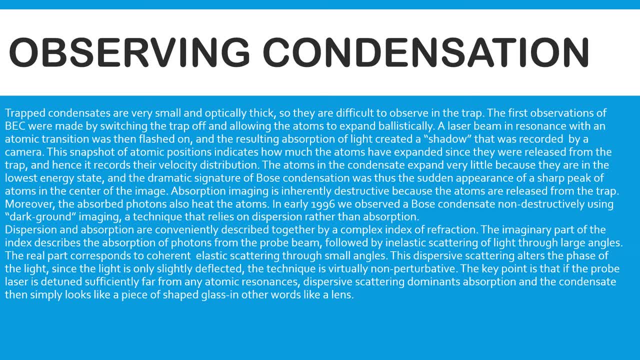 reduced to maintain evaporation at the edge of the cloud Observing Condensation Trap condensate are very small and optically thick so they are difficult to absorb in the trap. The first observations of BEC were made by switching the trap off and allowing the atoms to expand ballistically. 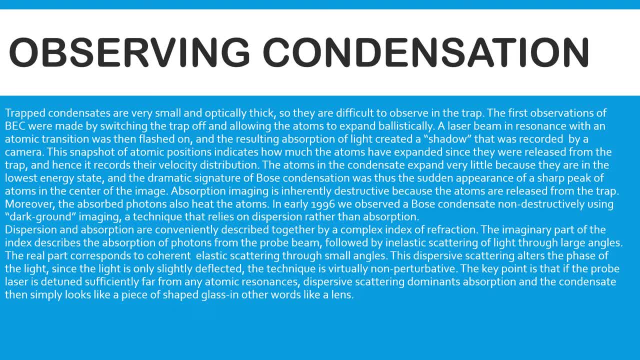 The laser beam, in resonance with an atomic transition, was then flashed on, and the resulting absorption of light created a shadow that was recorded by the camera. This snapshot of atomic position indicates how much the atom has expanded since they are released from the trap, And hence it records their velocity distribution. 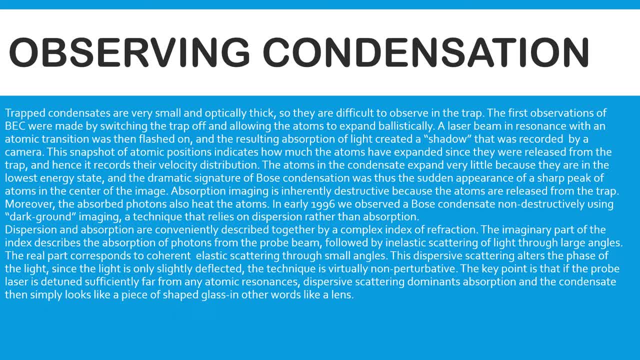 The atoms in the condensate expand very little because they are in the lowest energy state, And the dramatic signature of Bose condensation was thus the sudden appearance of a sharp peak of the atoms in the center of the image. Absorption imaging is inherently destructive. 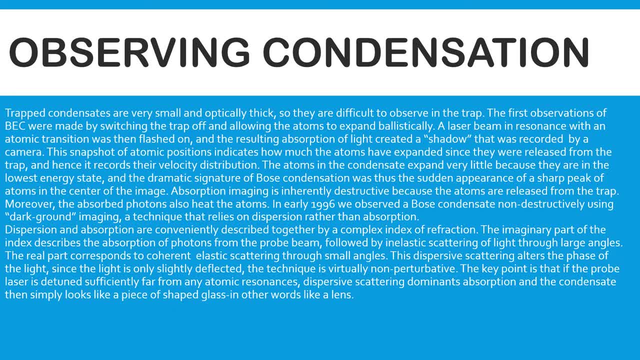 Because the atoms are released from the trap. Moreover, the absorbed photons also heat the atom. In early 1996, we absorbed a Bose condensate non-destructively using dark ground imaging, a technique that relies on dispersion rather than absorption. Dispersion and absorption are conveniently described together by a complex index of refraction. 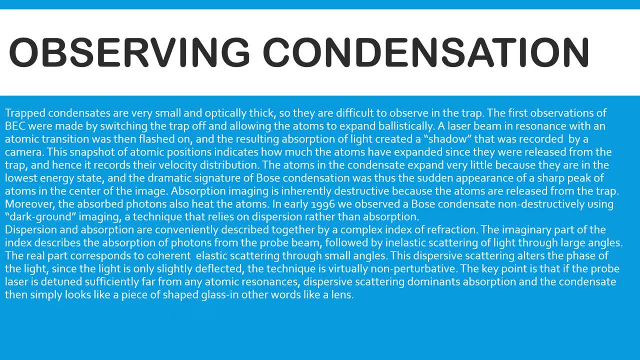 The imaginary part of the index describes the absorption of photons from the probe beam, followed by inelastic scattering of light through large angles. The real part corresponds to coherent, elastic scattering through small angles. This dispersive scattering alters the phase of the light, since the light is only slightly defected. 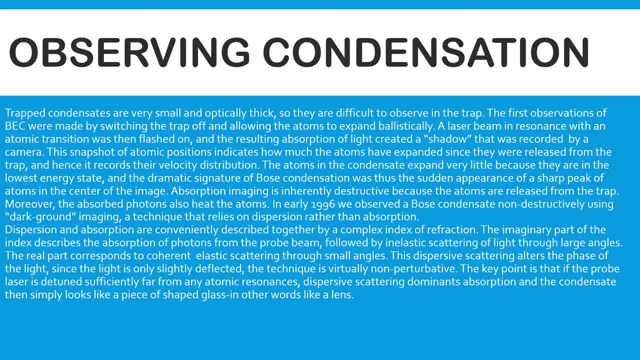 The technique is virtually impossible. The key point is that if the probe laser is detuned sufficiently far from any atomic resonance, dispersive scattering, dominant absorption and the condensate then simply look like a piece of shape glass, in other words, like a lens. 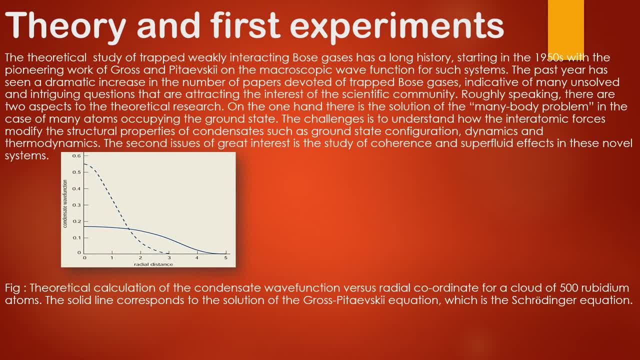 Theory and first experiments. The theoretical study of trap weakly interacting Bose gases has a long history, starting in 1950s with the pioneering work of Goess and Petayevsky on the microscopic wave function for such systems. The past year has seen a dramatic increase in the number of papers devoted to trap Bose Gases, indicative of many unsolved and intriguing questions that are attracting the attention of the public. 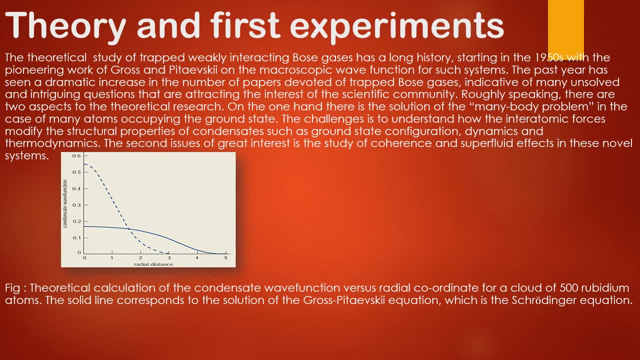 The theoretical study of trap weakly interacting Bose gases has a long history, starting in 1950s with the pioneering work of Goess and Petayevsky on the microscopic wave function. for such systems that are attracting the interest of the scientific community, roughly speak, there are to expect. 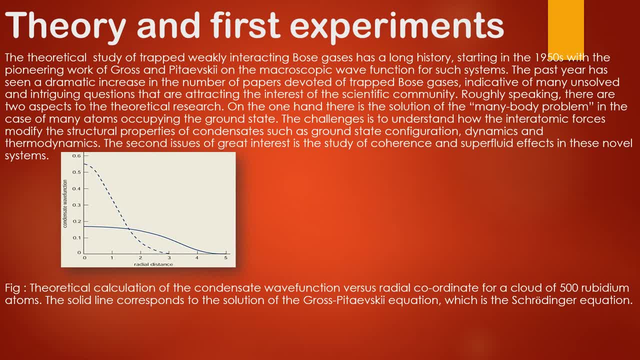 to the theoretical research. On the one hand, there is the solution of many body problems. in the case of many atoms occupying the ground state, The challenge is to understand how the interatomic forces modify the structural properties of the condensate, such as ground. 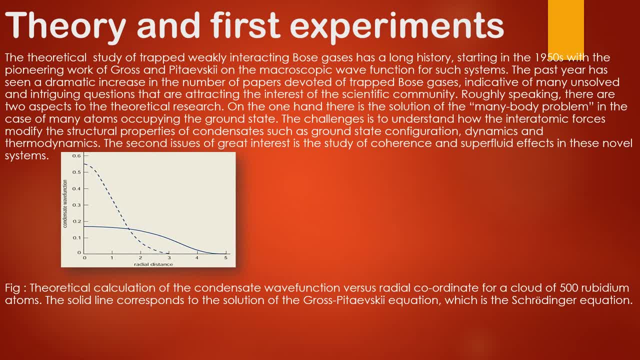 state configuration, dynamics and thermodynamics. The second issue of great interest is the study of coherence and superfluid effect in this novel system. As you can see, there is a graph plot between condensate wave function and radial distance in which it is decreasing. Figure: theoretical calculation of the condensate. 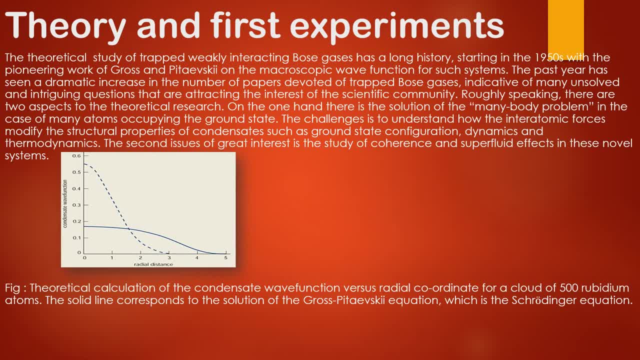 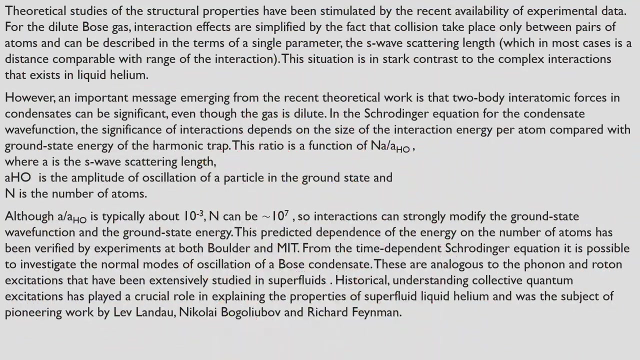 wave function versus radial coordinate for the cloud of 500-rub LG atoms, the solid line correspond to the solution of Gauss-Petovsky equation, which is the Scroudinger equation. Critical studies of the structural properties have been step by step, To be continued. 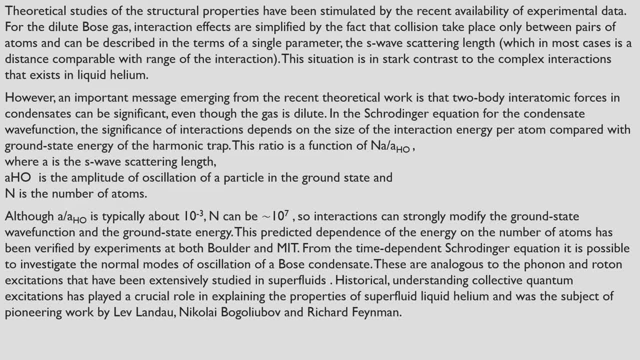 simulated by the recent availability of experimental data For the dilute-bose gas. interaction efforts are simplified by the fact that collisions take place only between pairs of atoms and can be described in terms of single parameter. The S-Wave scattering length, which is most case, is a distance comparable with the range. 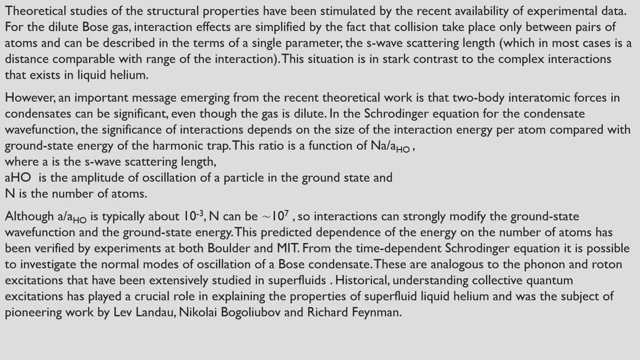 of interaction. This situation is in stark contrast to the complex interactions that exist in liquid helium. However, an important message emerging from the recent theoretical work is that two-body interatomic forces in condensate can be significant even though the gas is dilute. 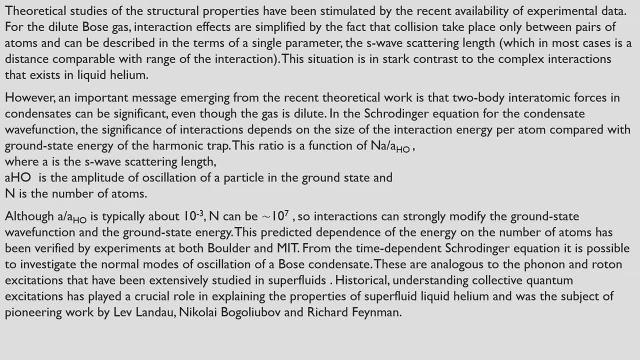 In the Schrodinger equation for the condensate wave function, the significance of interaction depends on the size of interaction energy per atom compared with ground state energy of the harmonic trap. This ratio is the function of Na by AHO, where A is the S-Wave scattering length, aho is 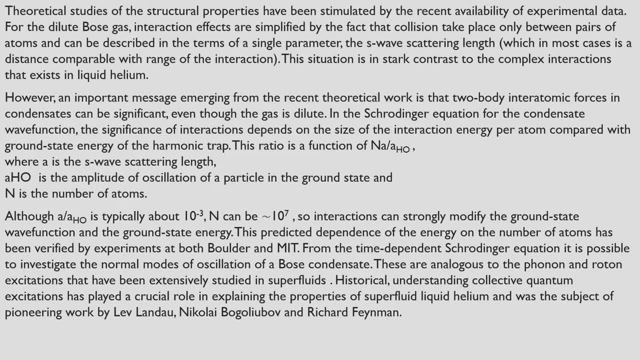 the amplitude of oscillation of a particle in the ground state and n is the number of atoms. Although A by A is the number of atoms in the ground state, the ratio of N to A is the number of atoms 4. 6.. 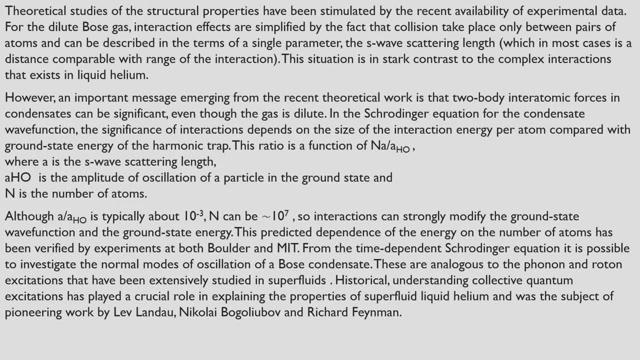 7., 8., 9., 10., 12., 12., 14., 15., 30. 27.. HO is typically above 10 to the power minus 3 and can be approximately 10 to the power 7. 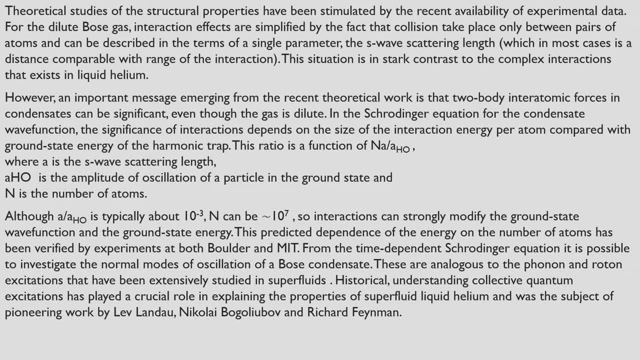 so interaction can strongly modify the ground state wave function and the ground state energy. This prediction dependence of the energy on the number of atoms have been verified by experiments at both borders and MIT. From the time dependent credential equation, it is possible to investigate the normal modes of oscillation of a Bose condensate. These are analogous to the phonon and 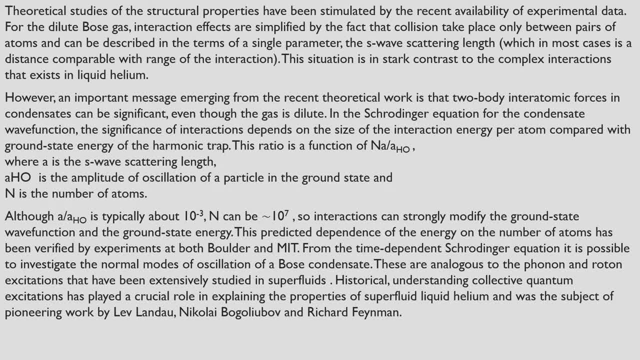 rotten excitation that have been extensively studied in superfluid. historically understanding collective quantum excitation. This equation has played a crucial role in explaining the properties of superfluid liquid helium and was the subject of pioneering work by Lev Lander, Nikolai Kololubo and Richard Ferrand. 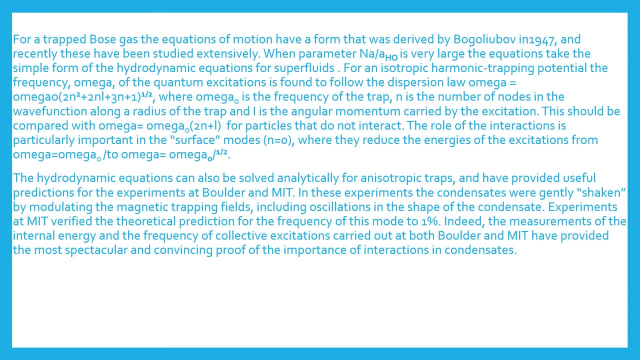 For a trapped Bose gas, the equation of motion have a form that was derived by Vogel's equation In 1947, and recently these have been studied extensively. When parameter NA by AHO is very high, the equation takes the simple form of the hydrodynamic equation. 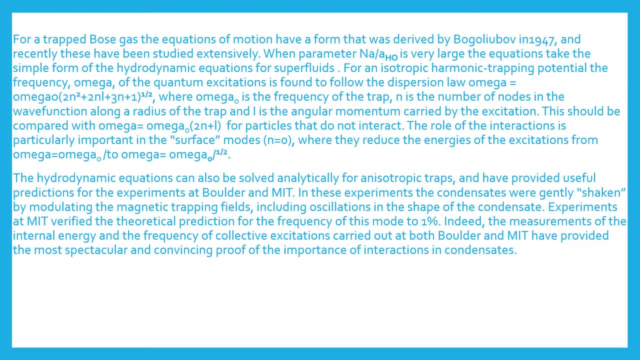 for the superfluid, For an isotopic harmonic trapping potential. the frequency omega of the quantum excitation is formed to follow the dispersant law. omega equals to omega month 2 n square by 2, and L plus 3n plus L to the power 1 by 2. well, omega not is the 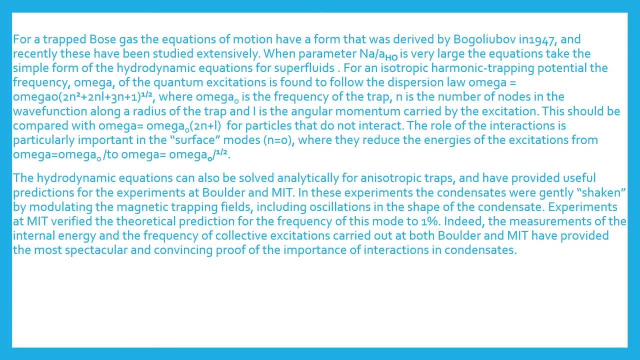 frequency of the trap, N is the number of nodes in wave function along a radius of the trap and L is the angular momentum carried by the excitation. This should be compared with omega equals to omega naught 2n and plus l. this should be compared to omega equals to omega naught 2n plus L and the 용 for yang level. 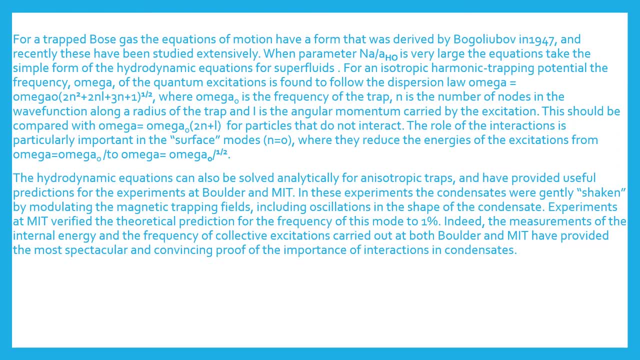 L for particles that do not interact. The role of the interaction is particularly important in the surface mode. N equals to zero. will they reduce the energy of the excitation from omega equals to omega naught by 2? omega equals to omega naught slash half. 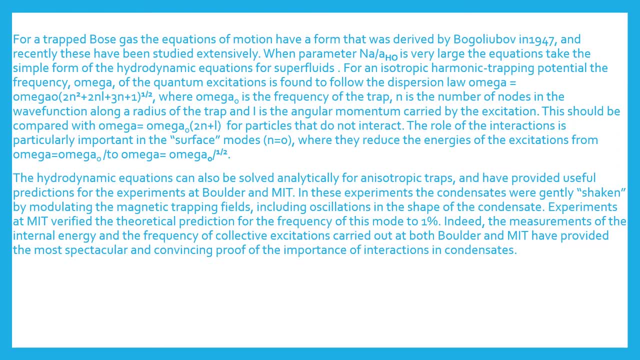 The hydrodynamic equation can also be solved analytically for an isotopic trap and have provided useful prediction for the experiment at Boulder and MIT. In this experiment, the condensates were gently shaken by modulating the magnetic trapping field, including oscillation. 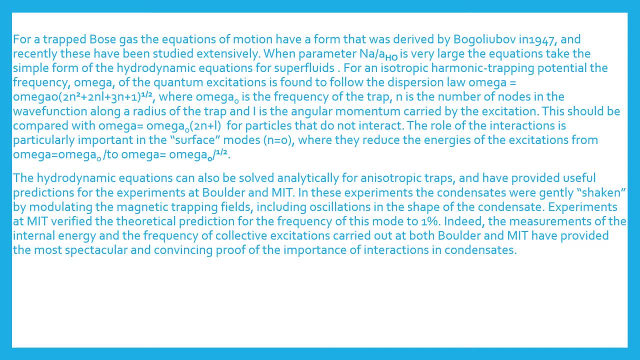 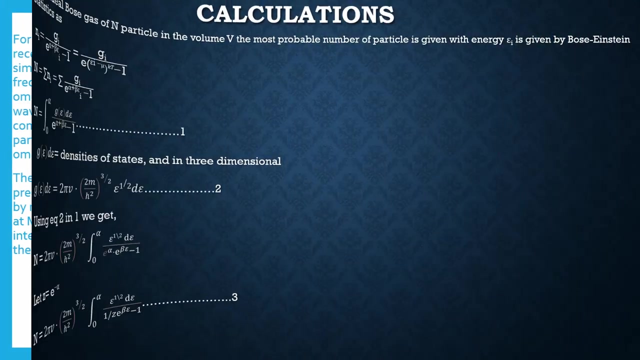 in the shape of condensate. Experiment at MIT verified the theoretical prediction For the frequency of this mode to 1%. indeed, the measurement of the internal energy and the frequency of collective excitation carried out at both Boulder and MIT have provided the most spectacular and convincing proof of the importance of interaction in condensates. 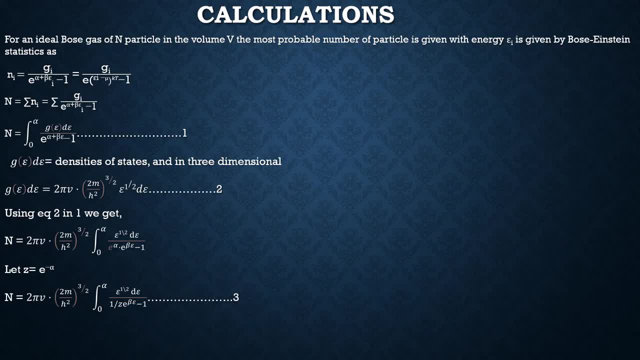 Calculation for an ideal Bose gas of N. For the frequency of N particles in volume V, the most probable number of particles is given with energy. epsilon i is given by Bose-Einstein statistics as: Ni equals to Gi by e to the power alpha plus beta. epsilon i minus 1 equals to Gi by e to the power epsilon i minus mu, kT minus 1.. 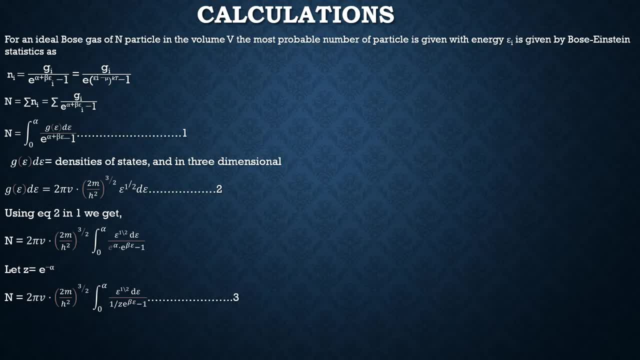 N equals to summation Ni. i equals to summation Gi by e to the power alpha plus beta epsilon i minus 1. N equals to 0 to alpha limits. gi epsilon d epsilon equals to e to the power alpha plus beta epsilon minus 1, which is equation 1. gi epsilon d epsilon equals to density of state N in 3.. 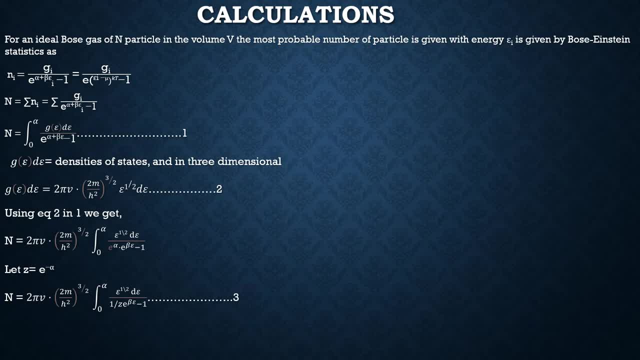 dimensional g epsilon. d epsilon equals to 2 pi v dot. 2 m by h square whole to the power 3 by 2 epsilon to the power 1 by 2 d epsilon. equation number 2.. Using equation 2 in 1, we get n equals. 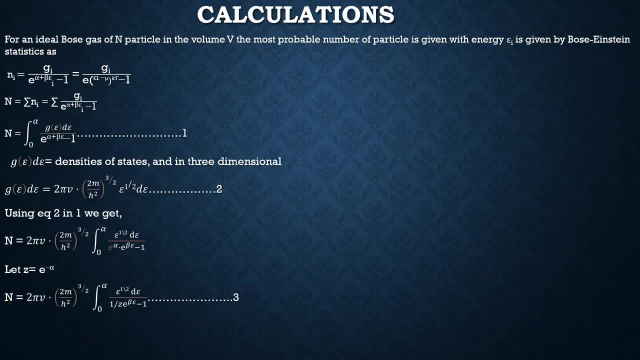 to 2 pi v dot 2. m by h square to the power 3 by 2. limits 0 to alpha integrating epsilon to the power 1 by 2 d epsilon by e to the power, alpha dot e to the power beta epsilon minus. 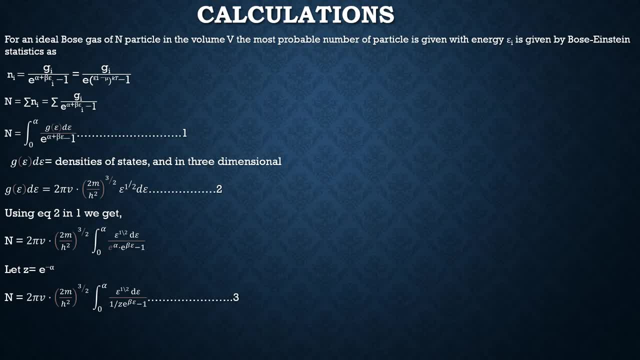 1. Let z equals to e to the power minus alpha, n equals to 2, pi v dot. 2 m by h square to the power 3 by 2. limit 0 to alpha integrating epsilon to the power 1 by 2 d epsilon by 1 by z e to the power, beta epsilon minus 1.. 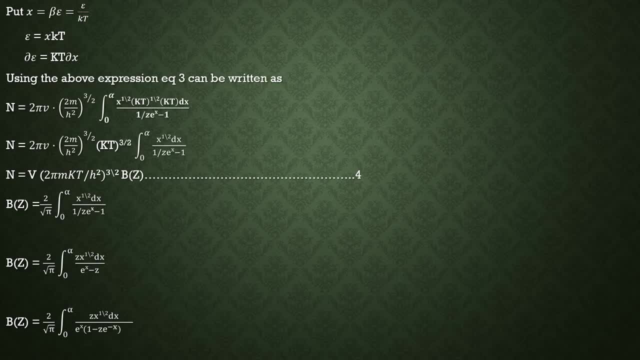 Put x equals to beta, epsilon equals to epsilon by kt. epsilon equals to x, kt d epsilon equals to kt dx. Using the above equation, 3 can be written as: n equals to 2, pi v, dot 2 m by h square to the power 3 by 2. 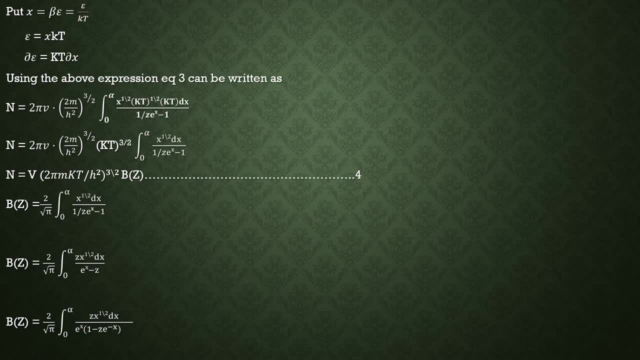 limit 0 to alpha. integrating x to the power 1 by 2 kt to the power 1 by 2 kt. dx by 1 by z e to the power x minus 1, and equals to two pi v dot to m by 1 by z e to the power x minus 1 and equals to 2 pi v. dot 2 m by h square to the power 3 by 2 kt to the power 3 by 2 element. 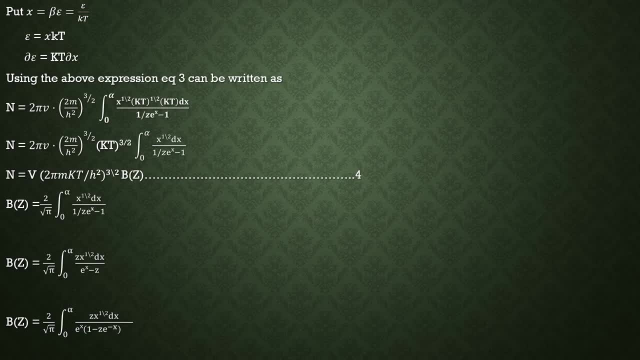 Integrating 0 to alpha x to the power 1 by 2 dx by 1 by z, e to the power x minus 1 n, equals to v, 2, pi, m, kt by h, square into: to the power 3 by 2 bz. 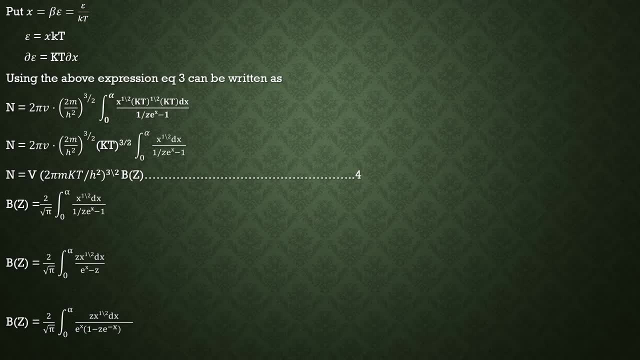 Equation number 4.. Bz equals to 2 by under root pi. 0 to alpha integrating x to the power 1 by 2, dx by 1 by z e to the power x minus 1.. Bz equals to 2 by under root pi 0 to alpha integrating z. 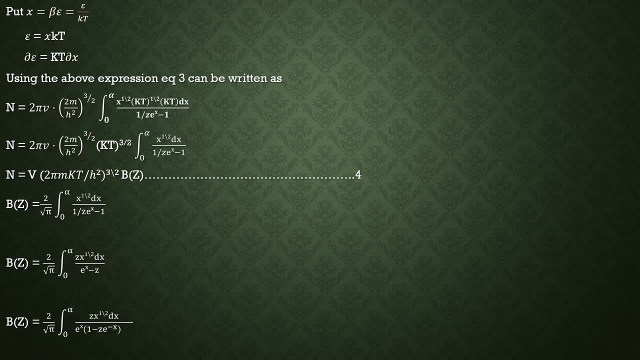 X to the power 1 by 2, dx by e to the power x minus z. Bz equals to 2 by under root pi 0 to alpha. integrating z, x to the power 1 by 2, dx by e to the power x into 1 minus z. e to the power minus x. 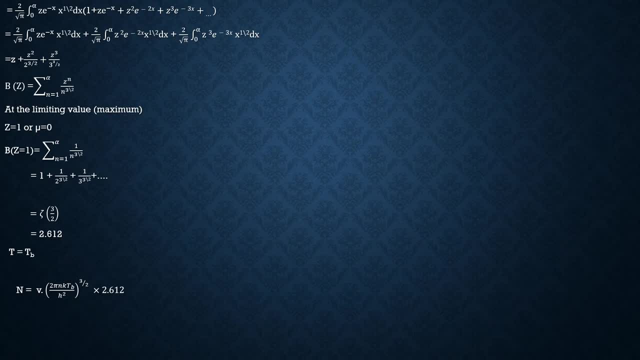 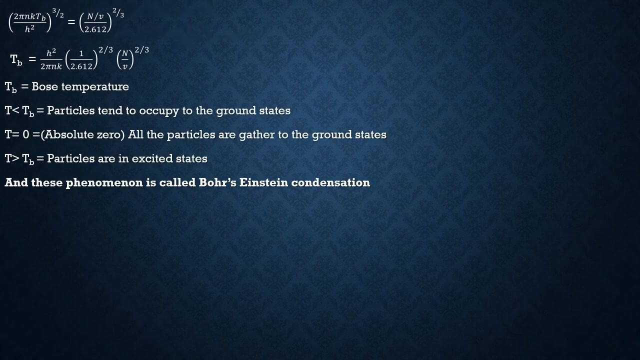 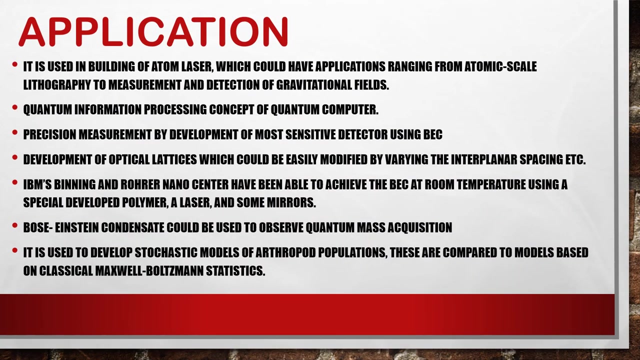 Bz equals to 2 by under root, pi 0 to alpha. integrating z, x to the power 1 by 2, dx by 1 minus z, e to the power x minus 1.. It is used in building of atom laser, which could have applications ranging from atomic 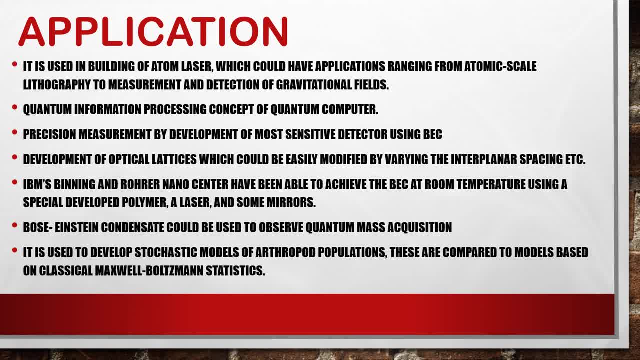 scale lithography to measurement and detection of gravitational fields. quantum information processing, concept of quantum computer precision, measurement by development of most sensitive detector using BC. development of optical latex which would be easily modified by varying the interplanar spacing as a drum. IBM's binding and rotor. 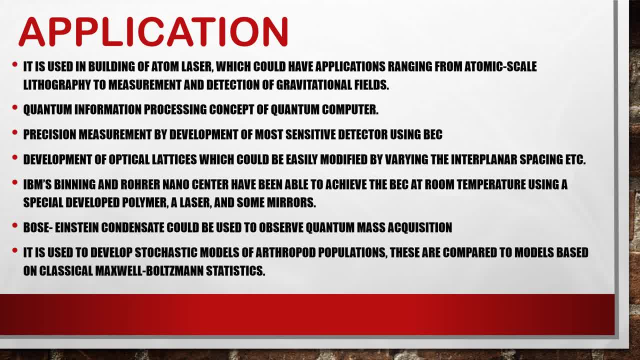 nanocenter have been able to achieve the BC at room temperature using a special development polymer or laser and some mirrors. Bose-Einstein condensate could be used to observe quantum mass acquisition is used to develop stochastic model of earthy port population. this are compared to: 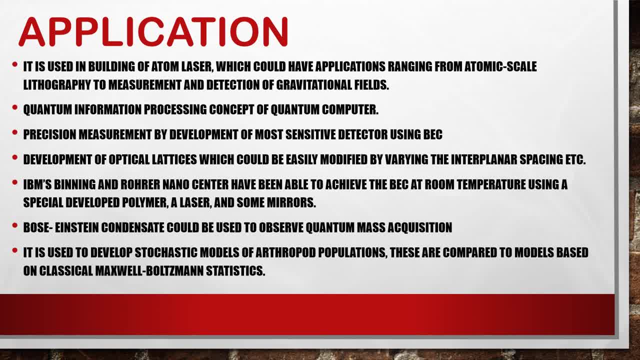 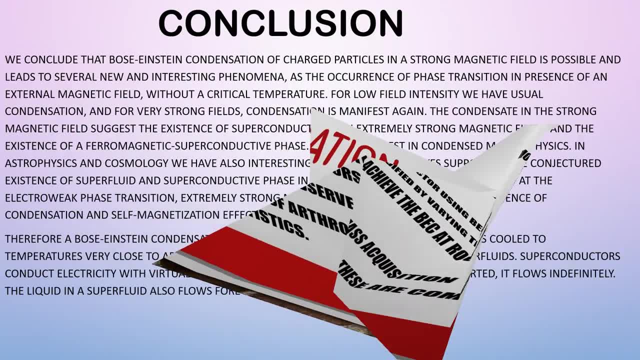 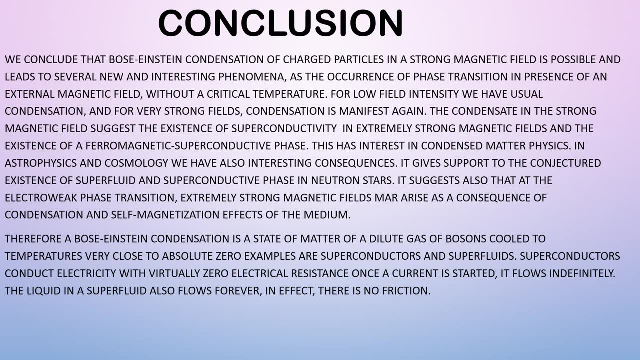 modern based on classical Maxwell-Boltzmann statistics. Conclusion: We conclude that Bose-Einstein condensation of charged particles in a strong magnetic field is possible and leads to several new and interesting phenomena, as the occurrence of phase transition in presence of an external magnetic field.